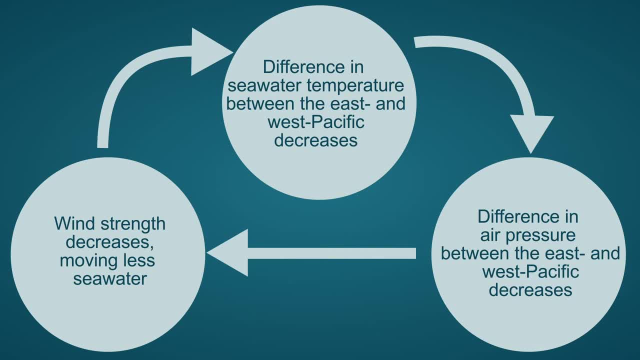 pacific decreases even more. In this way, the wind, sea temperature and air pressure influence each other. Although it is not known where it exactly starts, it is clear that if either the wind or the temperature of the sea water or the air pressure change, the other two are also affected and the 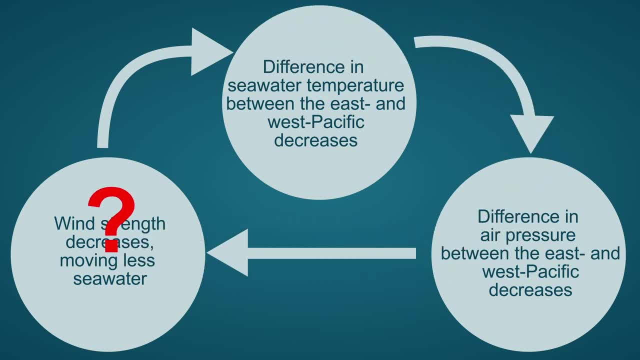 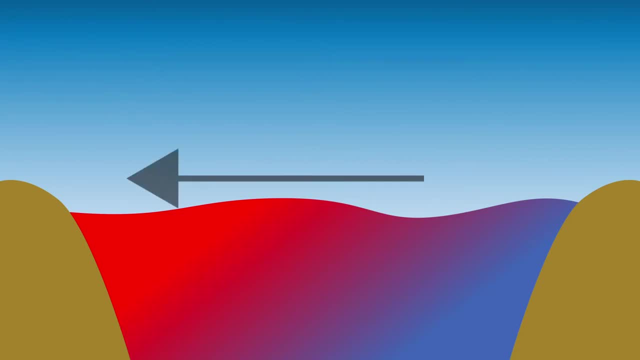 weather pattern changes. El Niño occurs about every two to seven years. The strength of the trade winds decreases, making the wind to the west less strong. As a result, the ocean water remains just west of south america and warms up there up to a maximum of six degrees celsius more than the 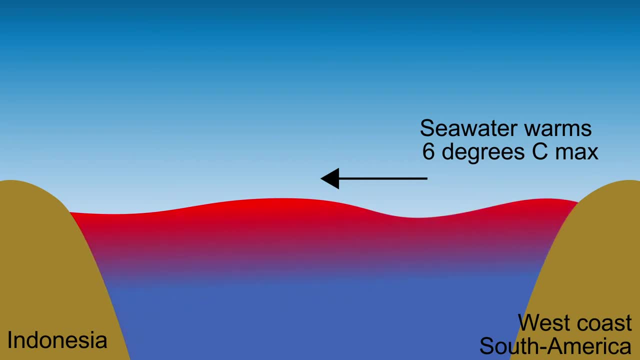 normal temperature. This creates a low pressure area and precipitation falls in a normally dry area, Because there is hardly any vegetation in this area. because normally there is no precipitation, the rain water is not retained and mudslides can occur. The warm ocean water. 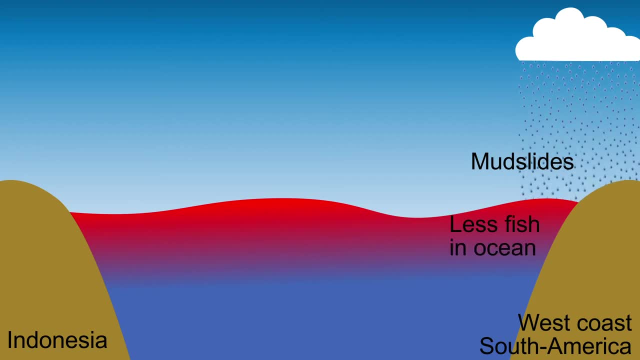 contained in the ocean water is not retained and mudslides can occur. The warm ocean water contains much less fish. South american fishermen noticed that this frequently occurs around christmas. They therefore called it El Niño, which is spanish for boy child, referring to the christ child. 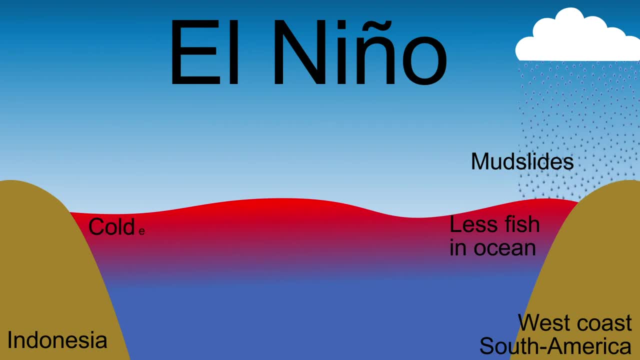 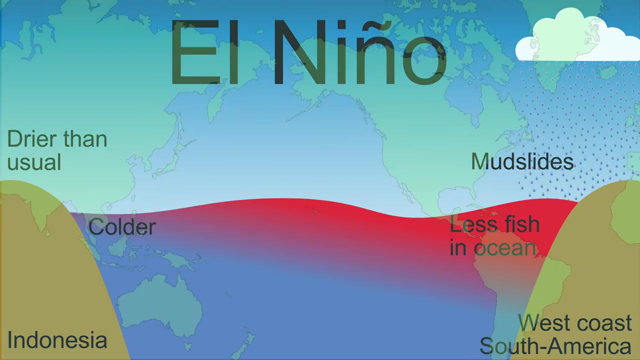 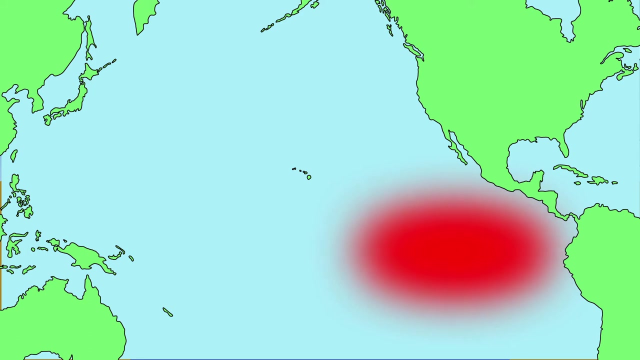 In the area around indonesia. the sea water is colder than normal. As a result, the air pressure increases and less water evaporates. This makes it a lot drier than normal. Agriculture and fisheries are thus greatly affected in both areas. If this situation continues for a long time, the warm sea water in the east and pacific ocean will eventually flow north and south. 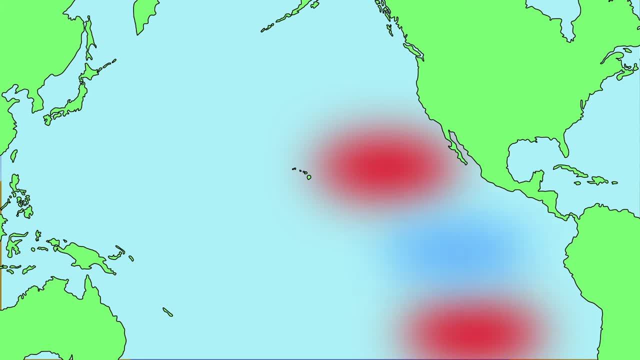 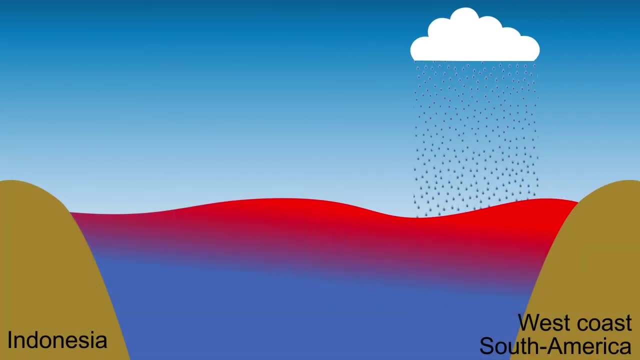 Deeper sea water, which is cooler, can now resurface. As a result, the surface temperature in the east and pacific ocean is getting colder and the weather is returning to the normal pattern. Sometimes, however, the sea water cools above average. in this area, This creates an extremely high pressure area. 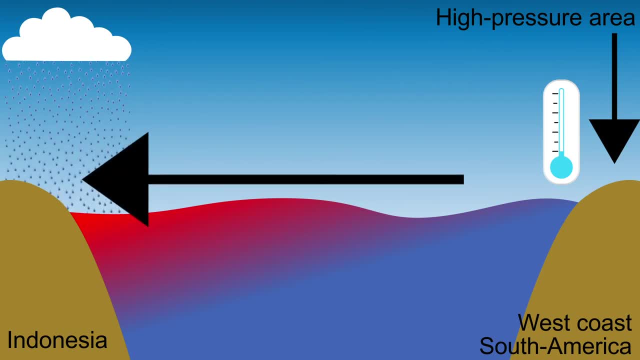 causing winds to the west to become stronger, More sea water to flow and lower the temperature flow west, more deep cold sea water to flow to the surface, creating a higher than normal temperature difference between the eastern and western Pacific. This will make it drier than normal in the eastern Pacific and even wetter than 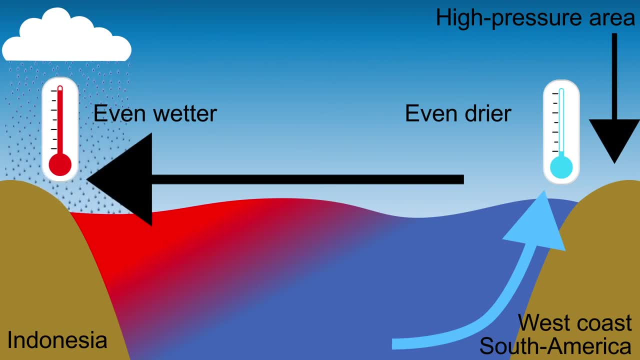 normal in the western Pacific. This opposite effect is called La Niña. This is Spanish for girl and thus the counterpart of El Niño, the boy. El Niño affects not only the Pacific around the equator, but many more areas, The warm sea.